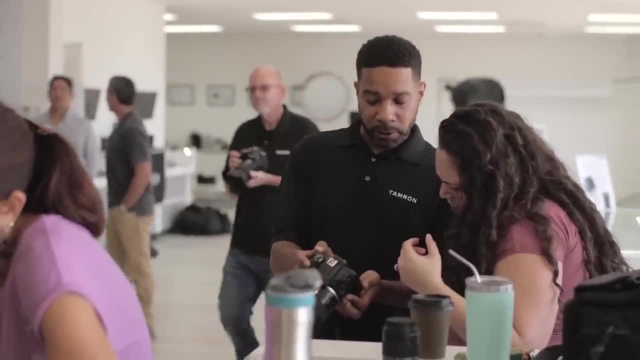 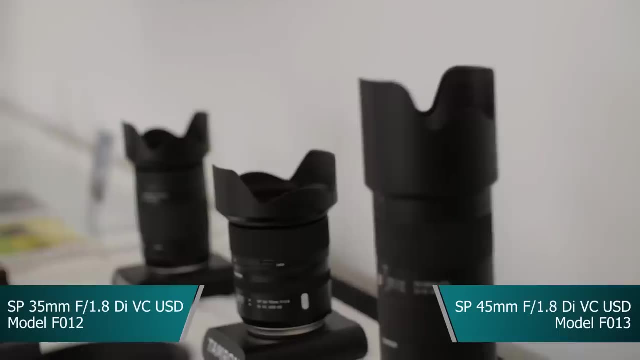 The kit lenses that come with most cameras can achieve photos where the background is blurry. Now, to achieve that effect in your photos, you want to use a fast aperture prime lens like the Tamron 35mm f1.8 or the Tamron 45mm f1.8 and shoot in an aperture priority at 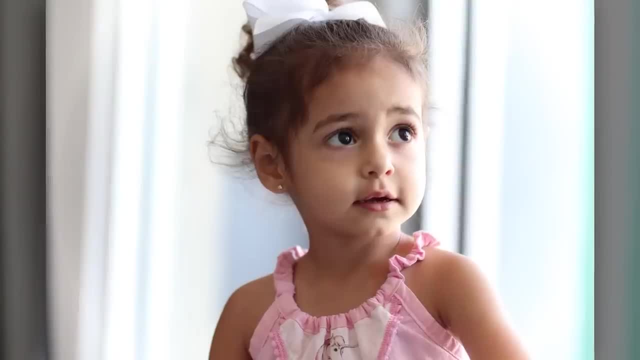 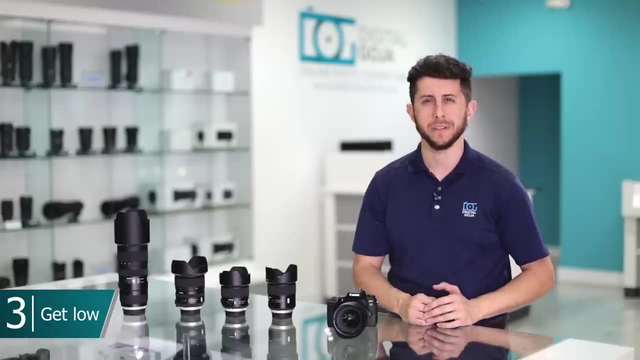 the largest aperture available. And remember, the closer you get to the subject, the more blur there will be in the background. When photographing children, get down on their level. Get close and try to shoot them at their eye level. Don't be afraid to get silly. 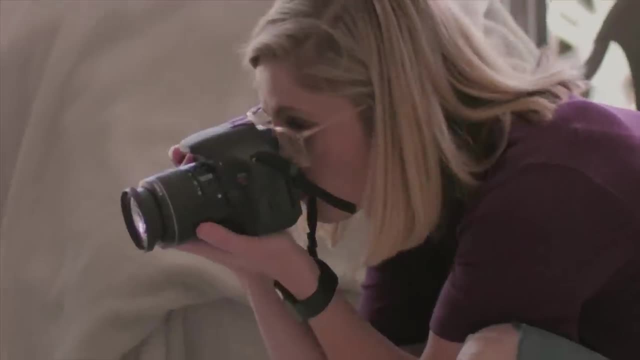 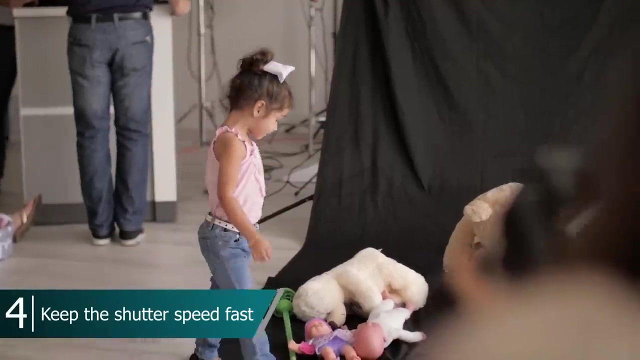 Have fun with the child and engage with them so that you can show their unique personality in the photo. To get great candids of your kids, keep your shutter speed fast. Kids move around fast and many moms get frustrated when they take photos of their kids and all. 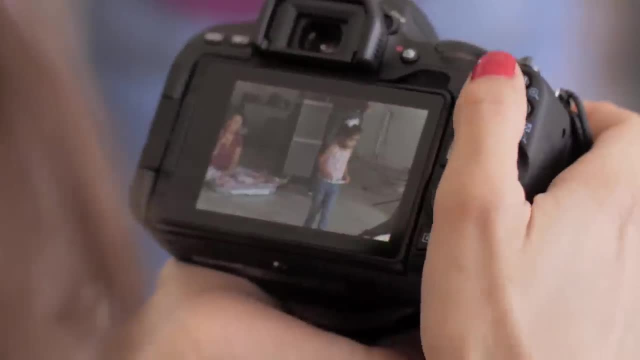 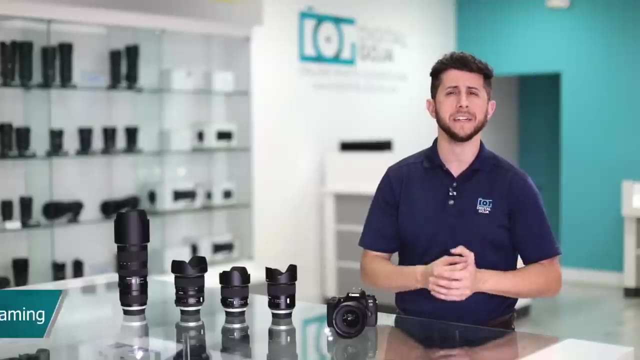 you see is a blur. Now. the easiest way to get them in action is to shoot in shutter priority mode and keep the shutter speed at 1, 2, 50th of a second. Be aware of all the elements in the frame. It's easy to get caught up in the moment and not notice what's in the frame. 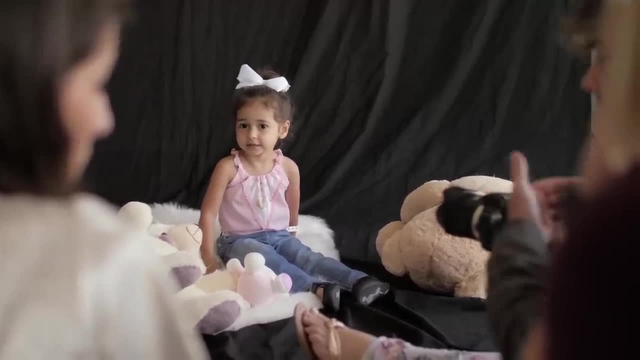 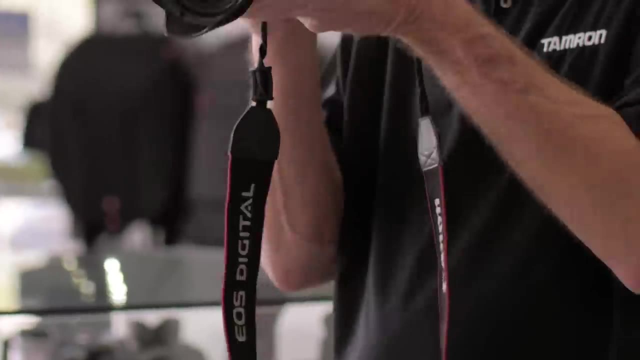 You don't want a tree limb coming out of their ear or a garbage can in the scene. Take your time, Set up the shot by choosing a location that looks good and makes the child feel comfortable. Don't be afraid to take a step to the left or to the right. 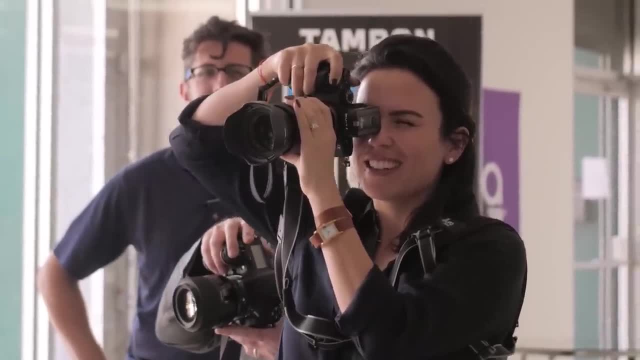 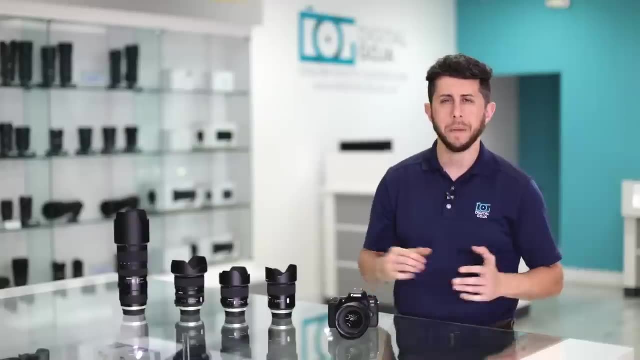 If you're shooting with a telephoto zoom lens like the Tamron 70-200 f2.8,, make sure to give yourself plenty of room, since you won't be able to get as close to your subject. Remember, when photographing kids, the most important thing is to have fun and make your 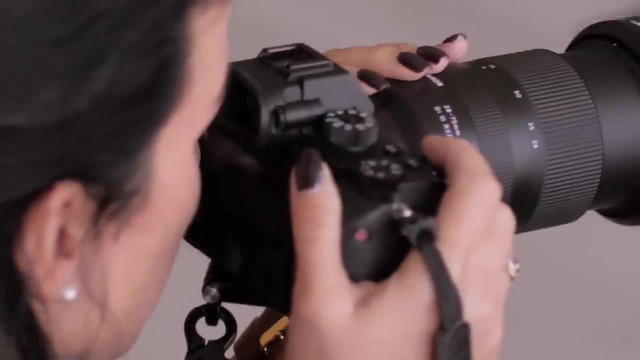 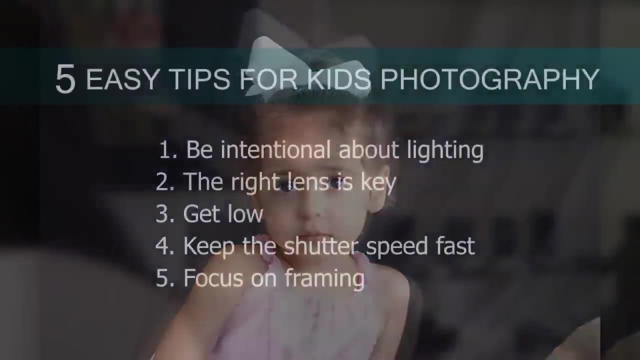 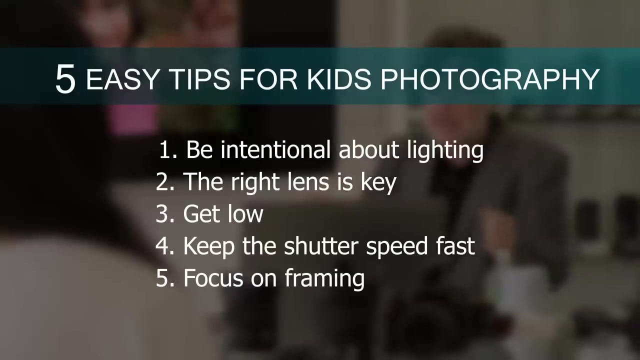 kid feel special. There are no bad shots. Just continue shooting. Even a photo of your kid crying could be a picture you treasure years down the line. Thanks again to Tamron and all the moms who participated, and especially Andre Constantini for sharing his insights on how to capture beautiful photos. 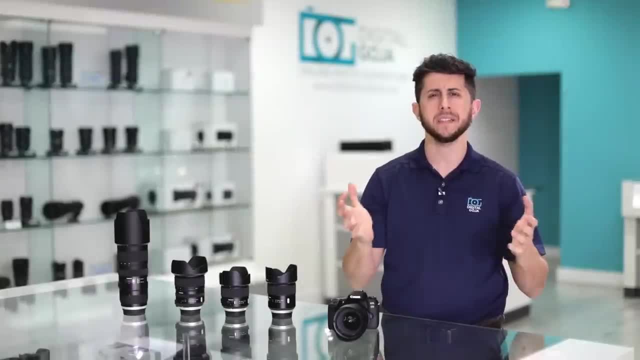 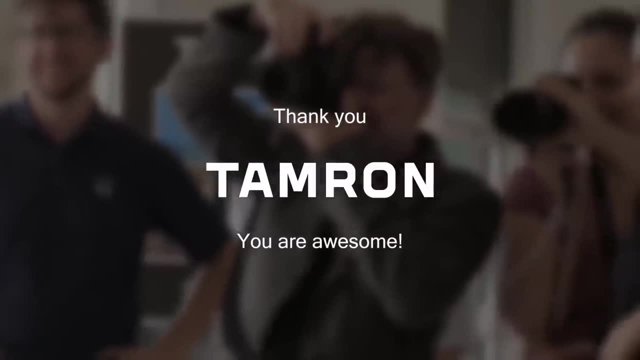 And thanks to you for watching. We're going to have more photo workshops in the future. Please let us know in the comments section below what type of photo workshops interest you, And we'll see you in the next video. Bye.